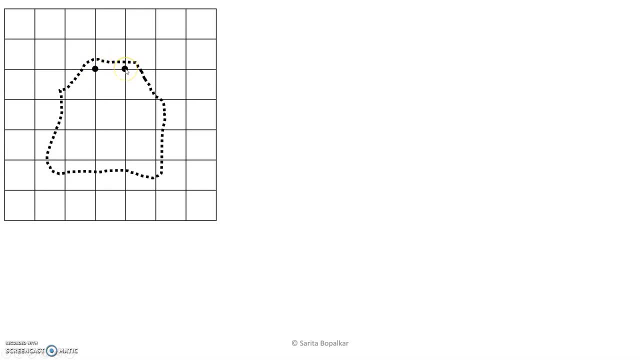 Like this, here the nearest grid point is this one, then here this one, now this is the nearest to these grid points. Like this, we will assign the grid points to the district boundary points and this technique is called as a re-sampling the boundary. 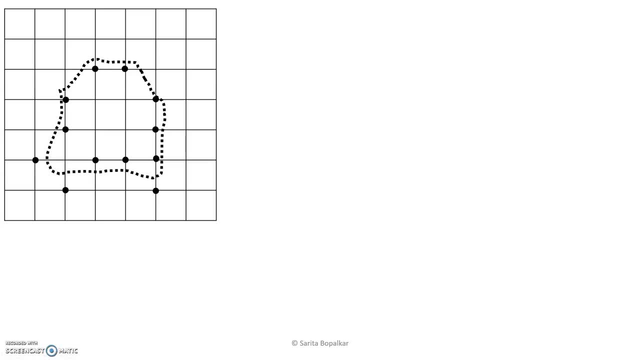 Then, to get a Chain Code, we need to decide a boundary. Now, let us see the direction scheme. It can be either 4-connectivity or 8-connectivity. 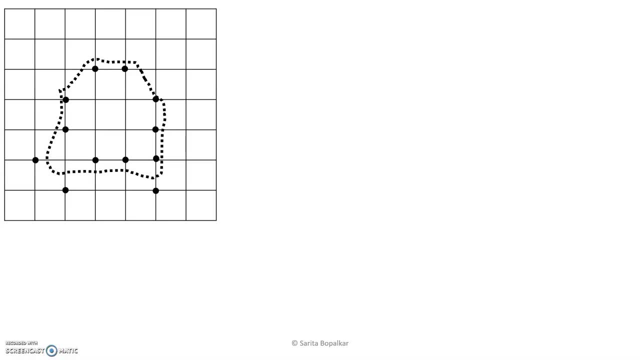 Here, we will use 8-connectivity. So, these are the 8-connectivity. If we start from this point, if your next pixel moves in this direction, we will represent by 0. If next pixel will move in this direction, we will represent by 1. Like this, 2, 3, 4, 5, 6, 7, according to the in which direction your next pixel is. So, let us decide. 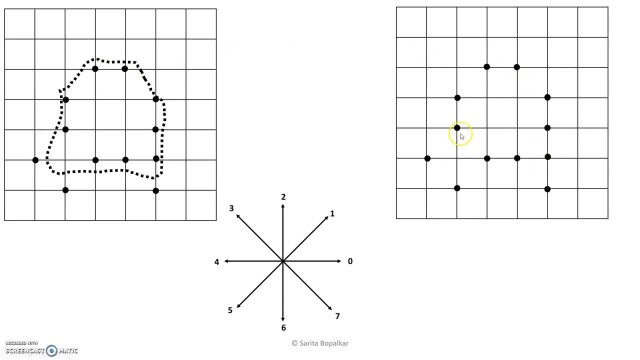 These are the grid points I have copied here. Now, let us decide the start point. Let this is our first start point. 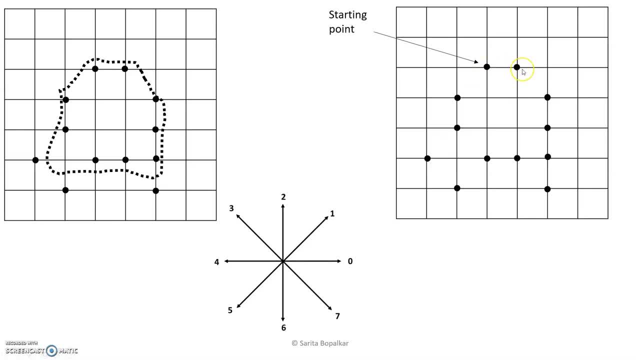 We will start from here, then the next grid point is this one. Now, check the direction. 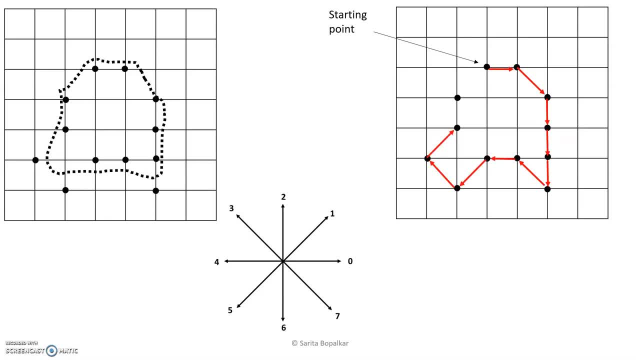 Like this, we will decide the next grid points. So, this is your boundary. 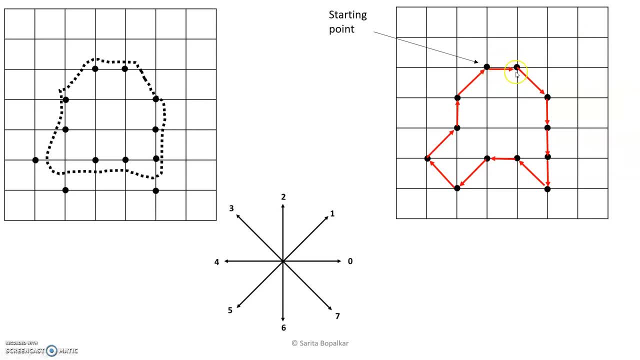 To represent the move from this grid point to this grid point, the direction is this one, which is represented by 0. 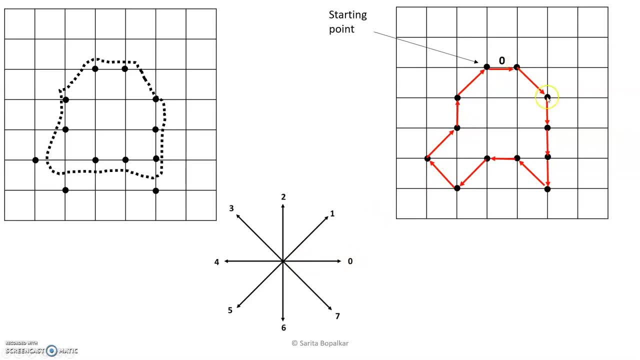 Now, here from this grid point, next point is in this direction and this direction is represented by 7. Like this, each direction we are representing by a number from this 8-connectivity. So, this is our chain code. 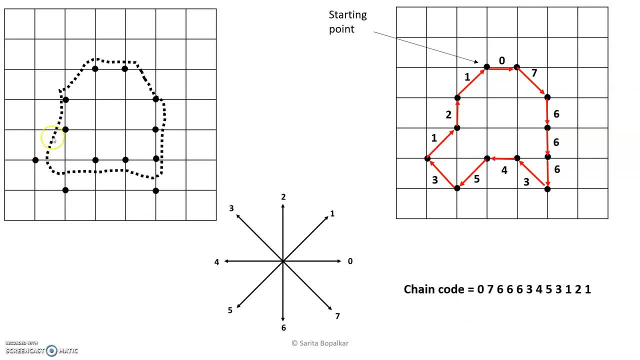 What we did here to obtain a chain code, we have given this district boundary points. Instead of obtaining a chain code from this district boundary point, we resampled it by using a grid scale and then we decided the sign convention to get a chain code. 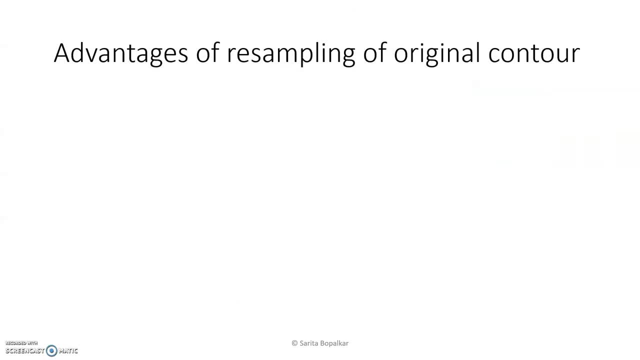 What is the advantage of this resampling? First advantage is it reduces the length of the chain code. Second one, we may get different chain code from the original boundary due to discretization process. 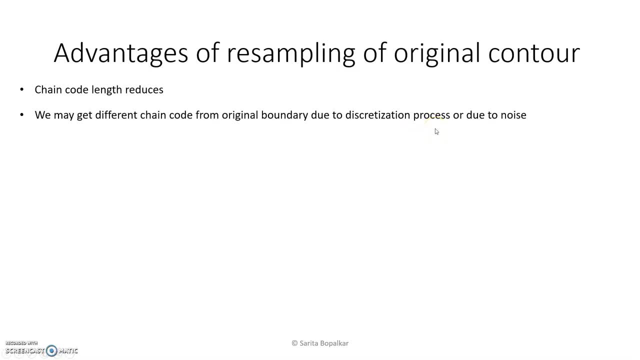 Or due to noise. So, when the boundary is discretized, there may be introduced some noise. 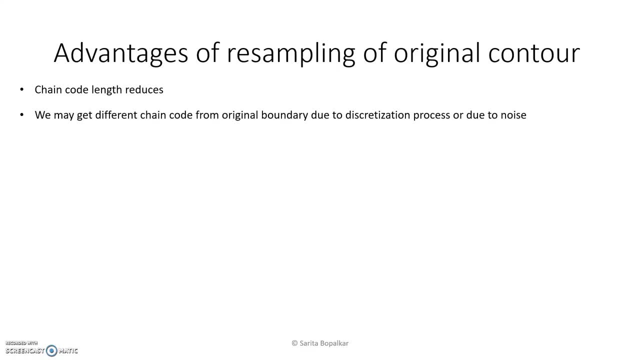 And if we are obtaining chain code from that original boundary, district boundary points, we may get different chain codes due to the noise. 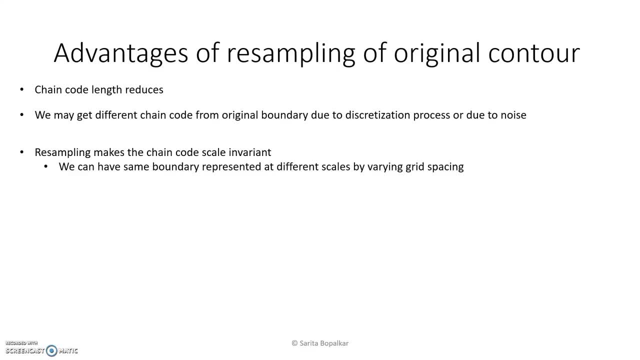 And due to resampling, this gets avoided. The most important advantage of this resampling is it makes the chain code scale invariant. 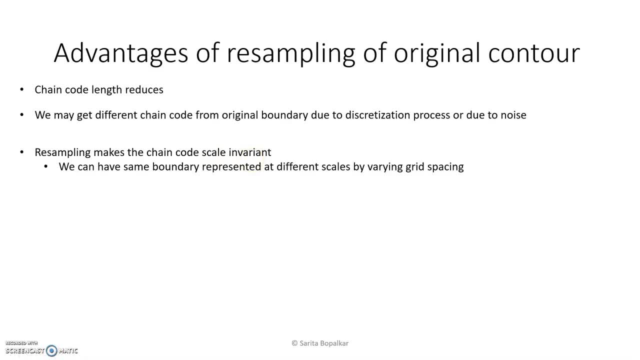 Means for same boundary point, we can change the grid scale to obtain a chain code. 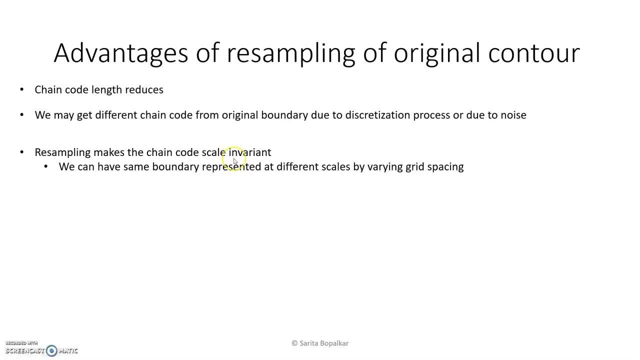 So, this chain code obtained a scale invariant but it is not a rotation invariant. Let us see the example. Now, these are the grid scales. 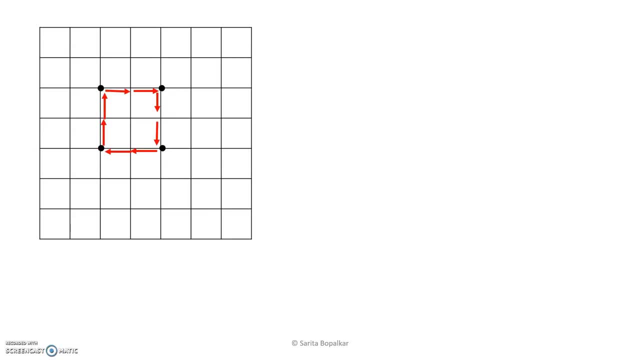 We will take one example of the boundary. So, these are the boundary points. 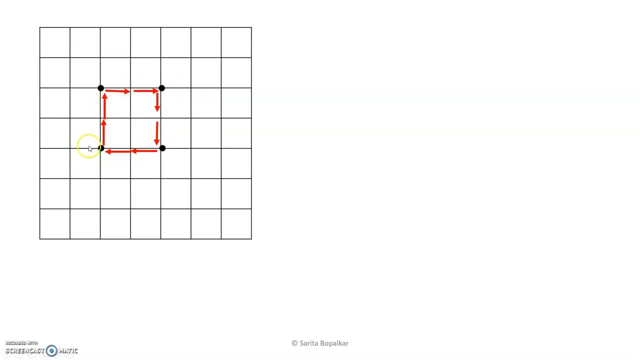 For simplicity, I have taken only four grid points as the boundary points. Now, the direction suppose this is our start point. 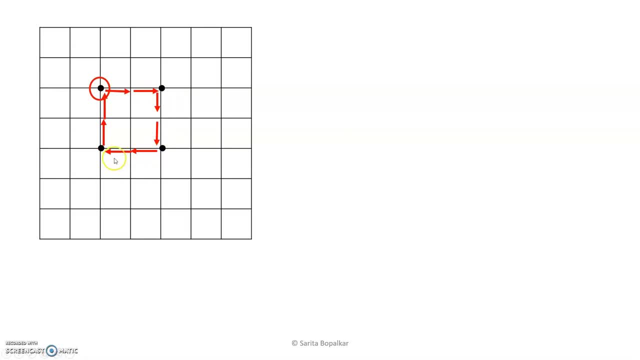 And our direction is this one. We will use the eight connectivity. So, this is represented by zero. This is represented by six. 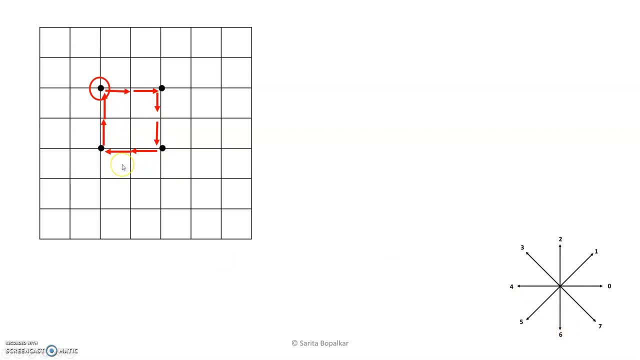 This one is represented by four. And two, two. 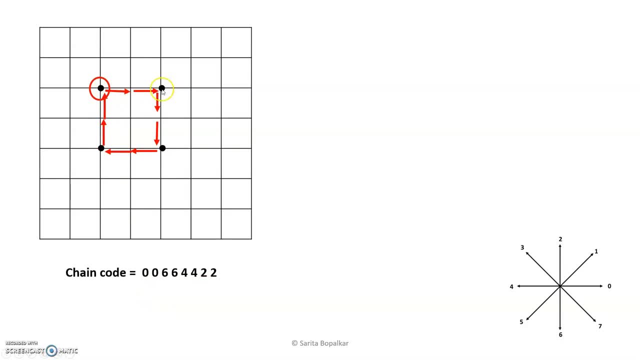 So, this is our chain code for these grid points. 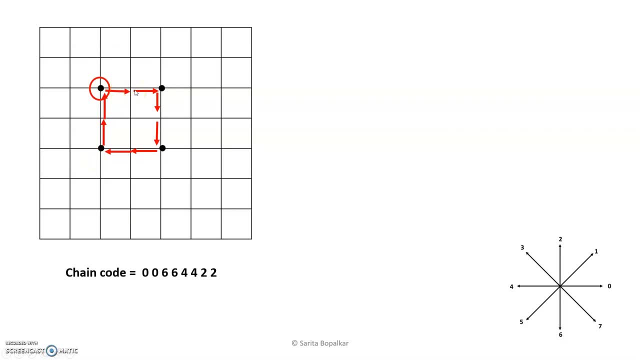 Now, we will rotate this grid points by 45 degree. Now, what is our chain code? 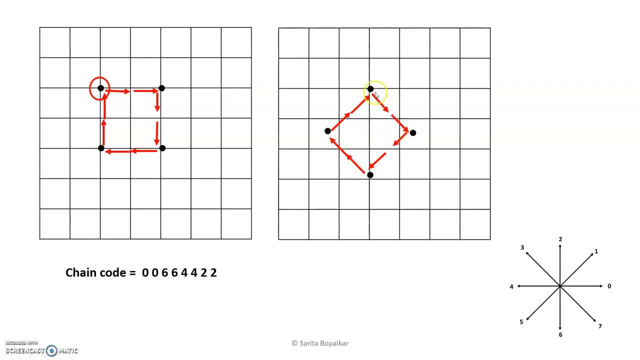 The direction changes. So, this is represented by seven. 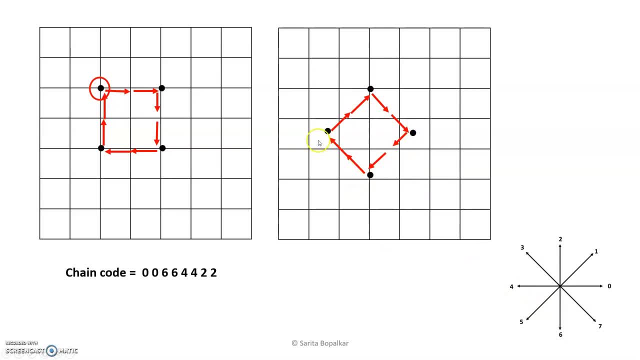 This one is represented by five. This direction is represented by three. 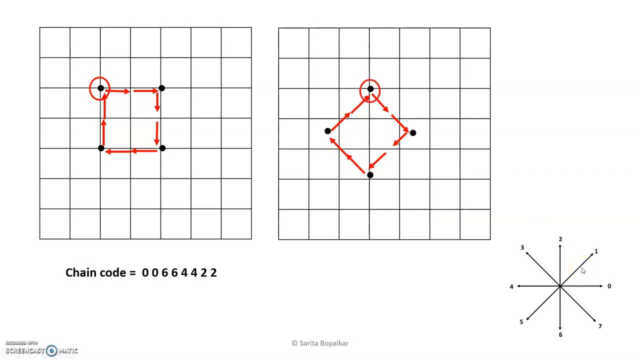 And this direction is represented by one. So, this is our start point. Your chain code is 77553311. 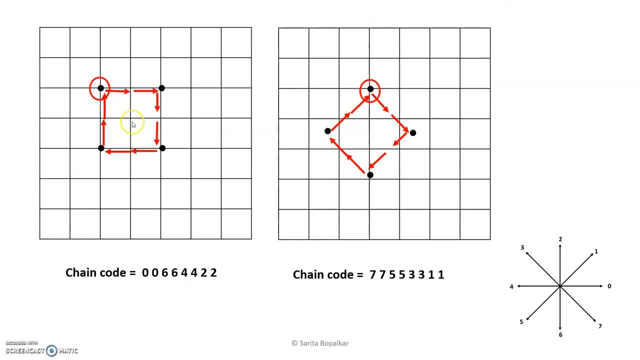 So, you will get the two different chain codes for the same boundary when we rotated it by 45 degree. So, we can say here that this chain code is not rotation invariant. 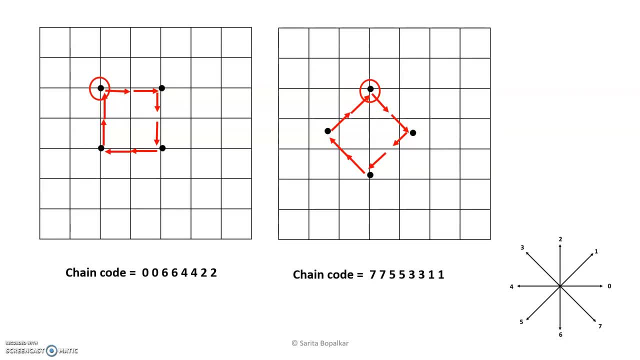 From this boundary representation, our objective is we want to find a descriptor. And this descriptor is compared with the descriptor stored into the machine. 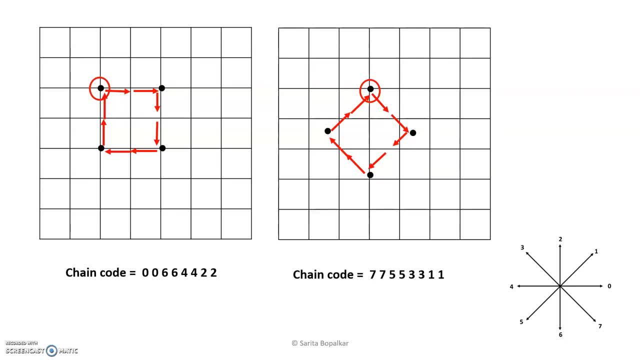 And if match is found, we can recognize the object. For that, our descriptor should be translation, scale, and rotation invariant. 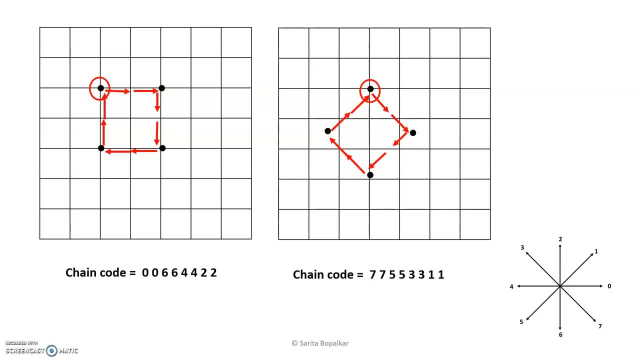 And to obtain that descriptor, our representation should be scale, translation, and rotation invariant also. So, this chain code, we studied that it is a scale invariant. 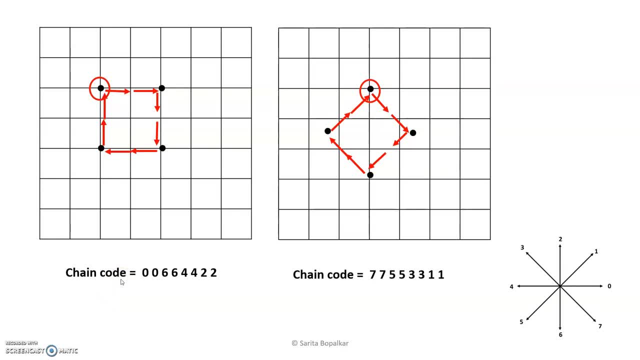 But to make it rotation invariant, we need a differential chain code. So, instead of obtaining the chain code from these grid points, we will obtain the differential chain code to make our code rotation invariant and scale invariant and translation invariant. 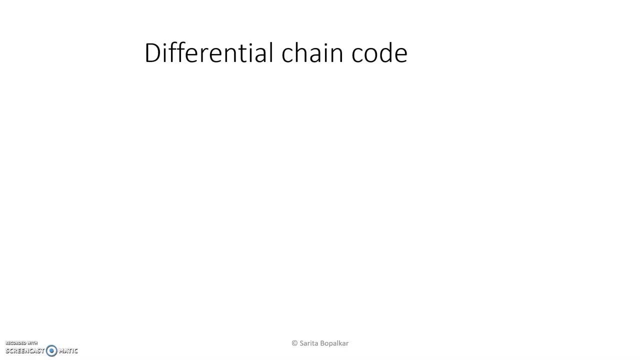 So, we will see how to obtain a differential chain code. This is our grid boundary points. This is the grid boundary points. This is the grid boundary points rotation after 45 degree. 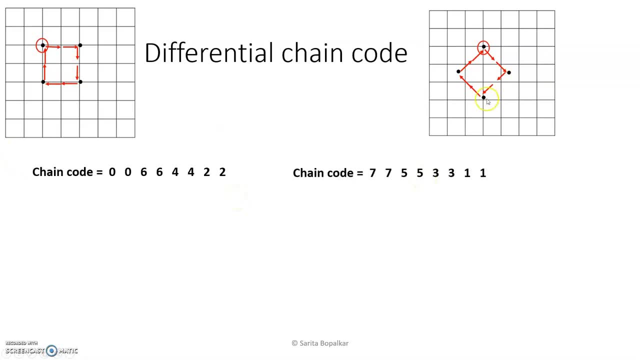 This is the chain code for these boundary points. This is chain code for these boundary points. 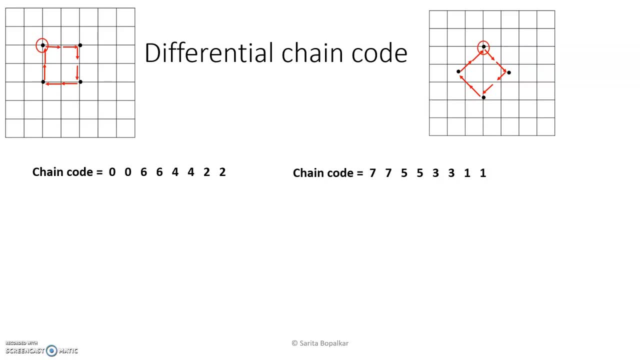 Now, let us see how to obtain a differential chain code. Take two subsequent codes. 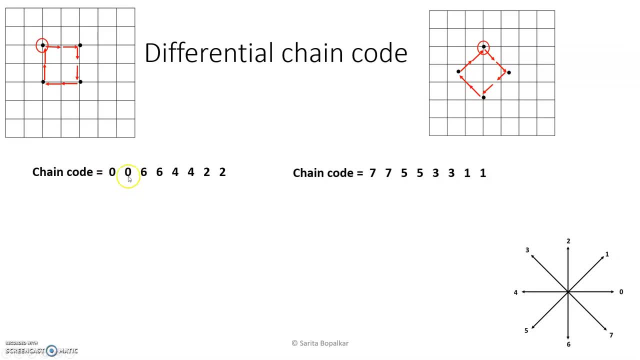 First, we will use the 8 connectivity. Now, take two subsequent codes. 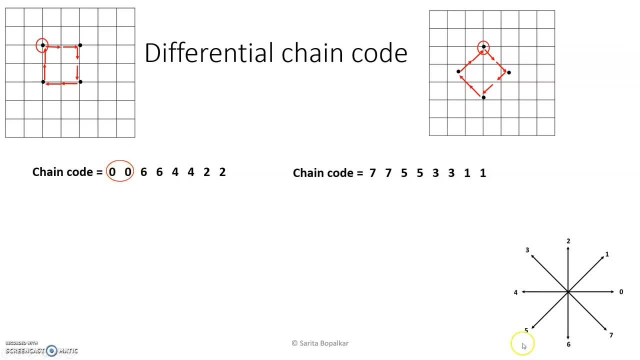 We will find out the number of moves in anti-clockwise direction in this 8 connectivity from first code to next code. 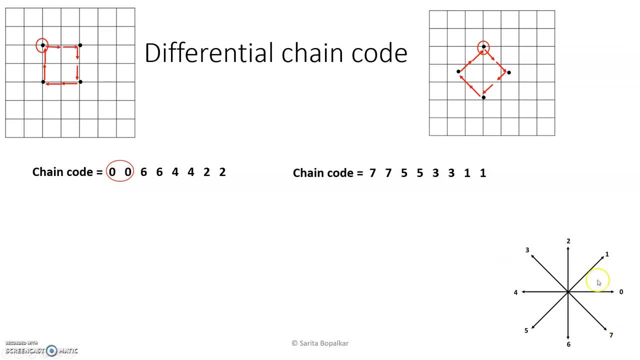 Now, here both the codes are 00. So, there is no need of move. 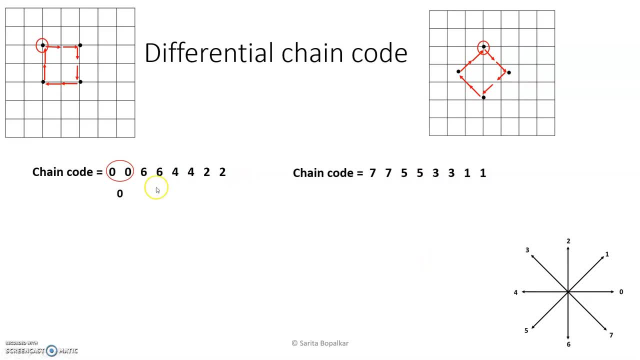 This is represented by 0. Now, next two subsequent points or numbers in a chain code is 0 to 6. So, we will find how many number of moves required to move from 0 to 6 in 8 connectivity. So, first move 1, 2, 3, 4, 5 and 6. 6 moves are required to move from 0 to 6 in a 8 connectivity. 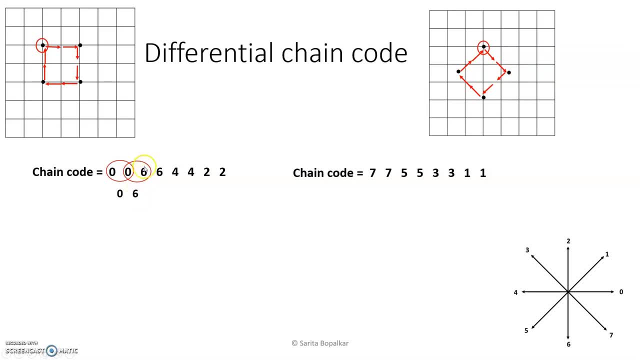 So, this represented by 6. Now, next is 6 to 6 means same number. The number of moves are 0. Then 6 to 4. 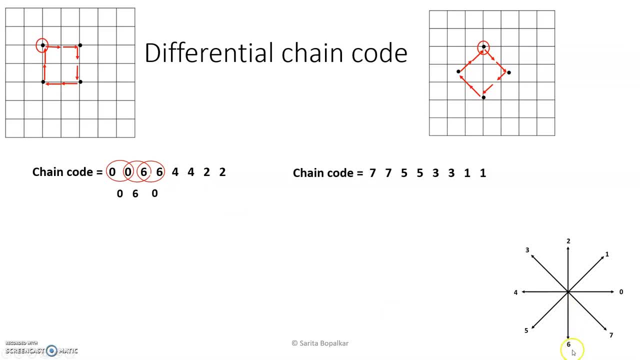 Now, let us see how many moves are required to move from 6 to 4 in anti-clockwise direction. 1, 2, 3, 4, 5, 6. 6 moves are required. 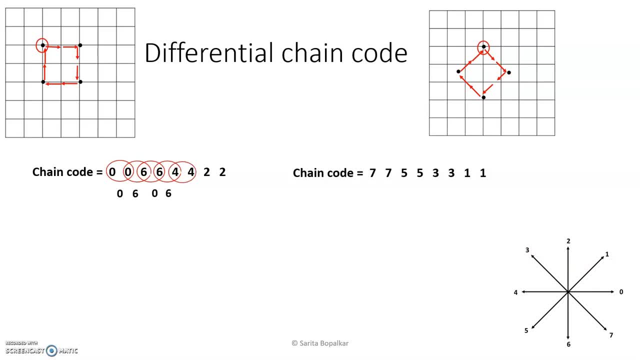 So, this represented by 6. Like this, 4 same number. 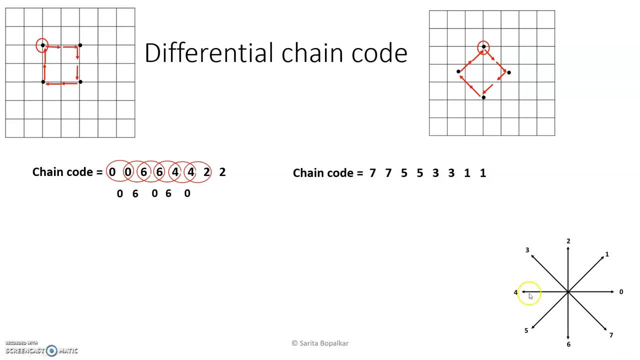 So, 0 moves. Then 4 to 2. How many moves are required in anti-clockwise direction? 1, then 2, 3, 4, 5, 6. 5, 6. So, 4 to 6. 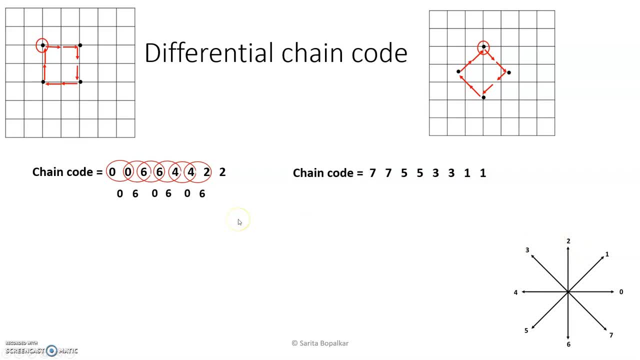 6 moves are required in 8 connectivity. Next two subsequent numbers are 2, 2. Then 0 moves are required. 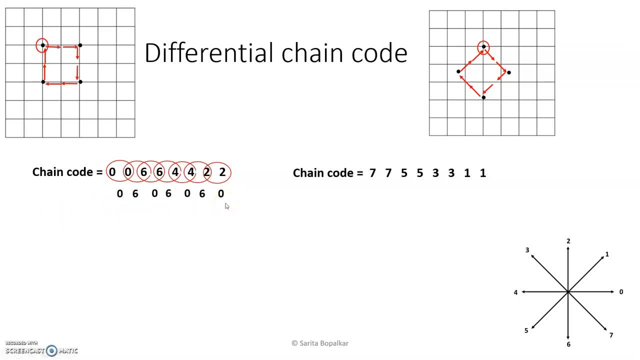 Like this, this is your differential chain code. How we obtained it? First, we get the first order chain code from the grid locations. By using either 8 connectivity or 4 connectivity. 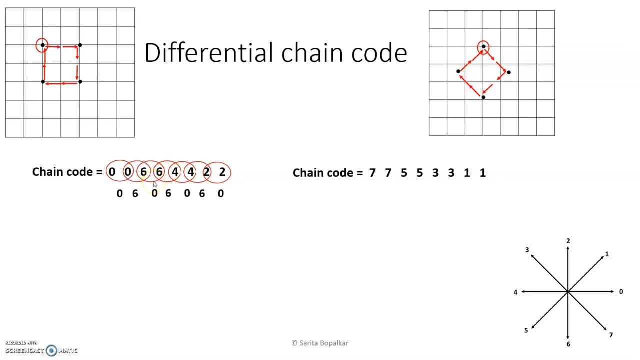 Most probably, we are preferring 8 connectivity. Then take two subsequent numbers in this code. 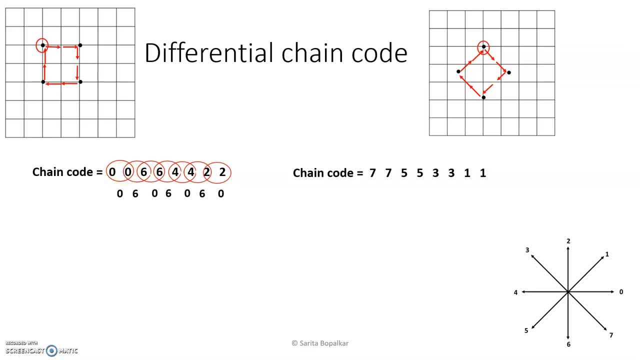 And find out the number of moves in anti-clockwise direction from first code to the next code. Like this, we will obtain the differential chain code. 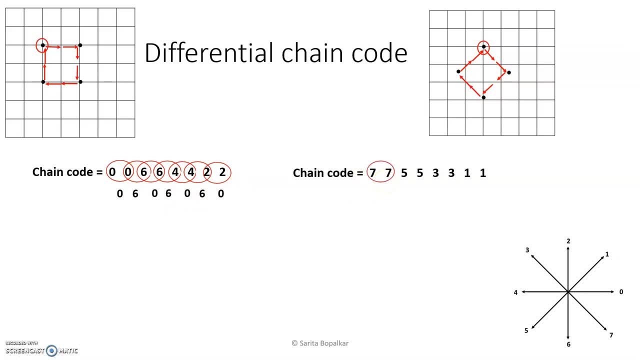 Now, for this one, 7, 7, same number. 0 moves. 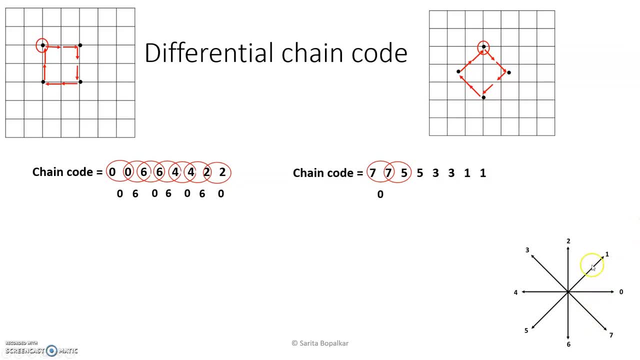 7 to 5. 1, 2, 3, 4, 5, 6. 6 moves. 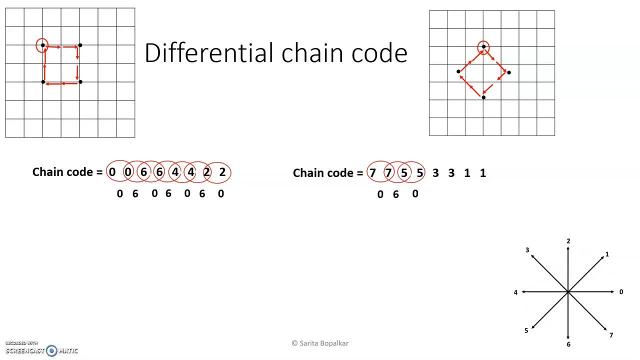 Then next subsequent numbers are 5, 5. 0 moves. 5 to 3. You can check how many moves required. It is 6. Then 3, 3. Same number. 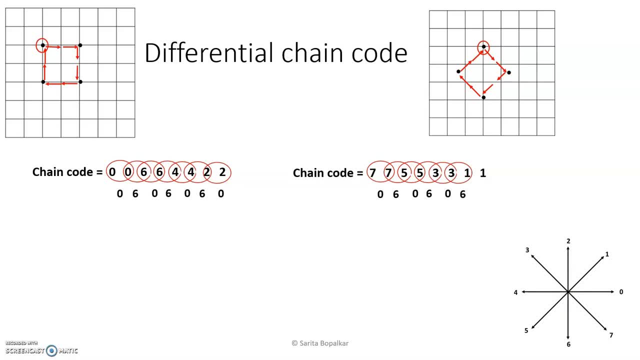 3, 1. Number of moves in anti-clockwise direction are 6. 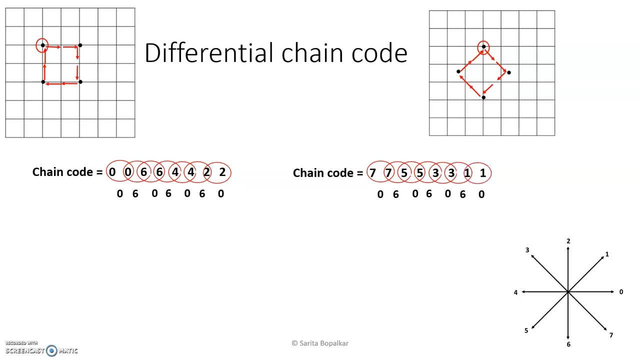 You can check it. And 1, 1, 0. 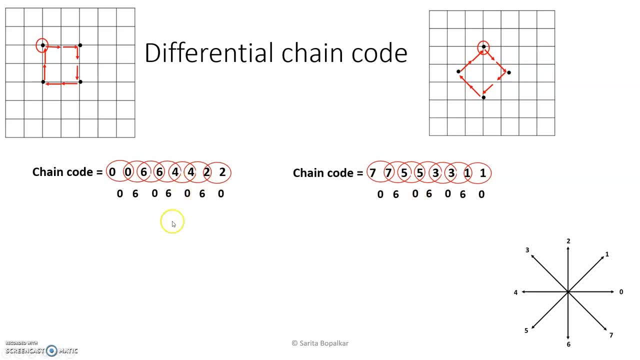 Now, if you observe this differential chain code for both the figures, it is same. So, even though your chain code is different due to rotation, but the differential chain code remains same. We are referring this differential chain code not as a chain, but as a cycle. Thus, this differential chain codes for both the after rotation and before rotation will get the same differential code. Thus, differential chain code makes the code rotation invariant. Thus, differential code is a rotation invariant, translation invariant and scale invariant. So, we obtained the representation which is rotation, translation and scale invariant. 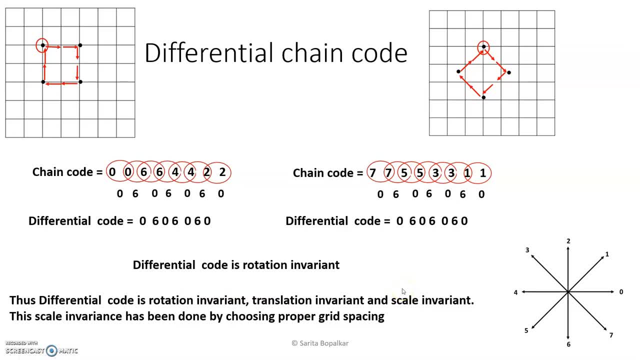 And from this representation, we can obtain a descriptor which we can compare with the stored descriptors for the recognition of the object. 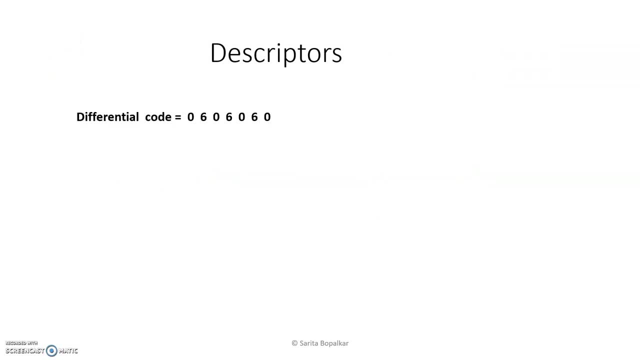 Now, how to obtain a descriptor? Differential chain code. We consider the differential chain code as a cycle instead of considering it as a chain. So, we will consider it as a cycle. Now, to explain how to obtain a descriptor, I will consider different chain code. It is easy to understand from another code. That's why I have taken different differential code. 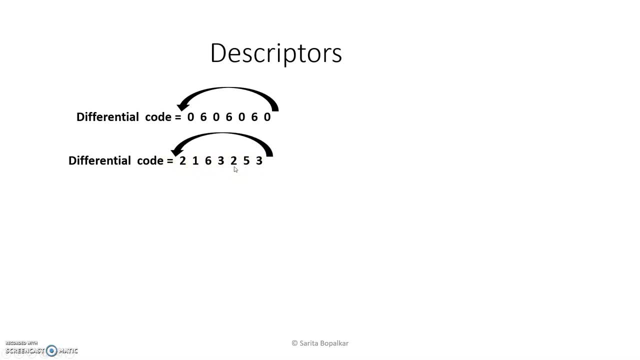 Now, this is one of the differential code. It is also we are considering the differential code as a cycle.